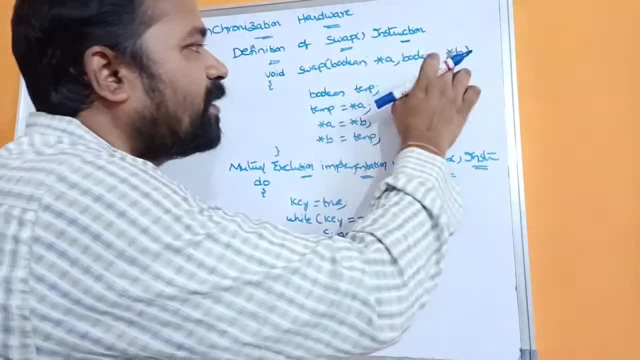 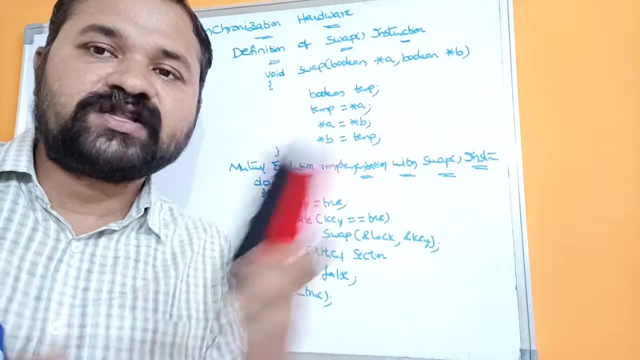 values may be either true or false. Here they are. of the types of pointer variables. That means we have to past their address to the corresponding Boolean values. Here we know pointer means we use call-by-reference. The major advantage of call-by-reference is: 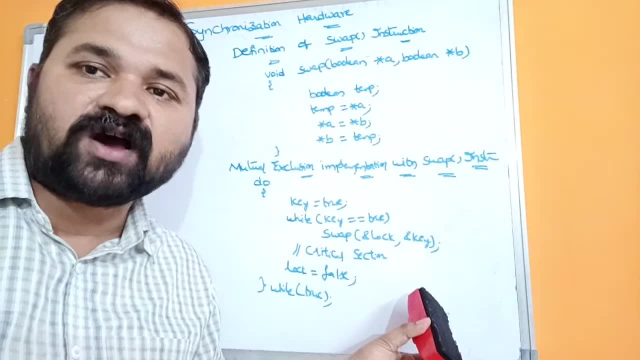 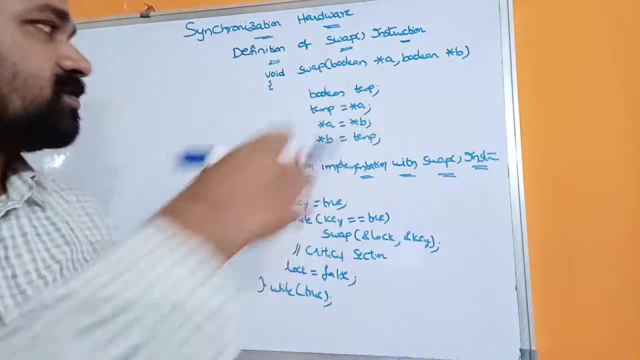 that if we perform any modification on actual arguments of the calling function, then those modifications will be affected on formal arguments of the call-to-function. So simple logic Boolean temp is used because it is running from and były entities. only We know how to swap two numbers. 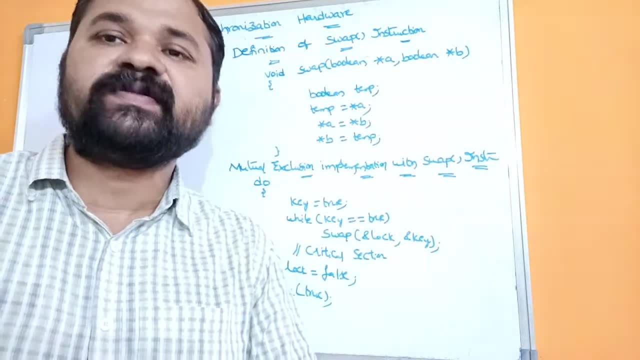 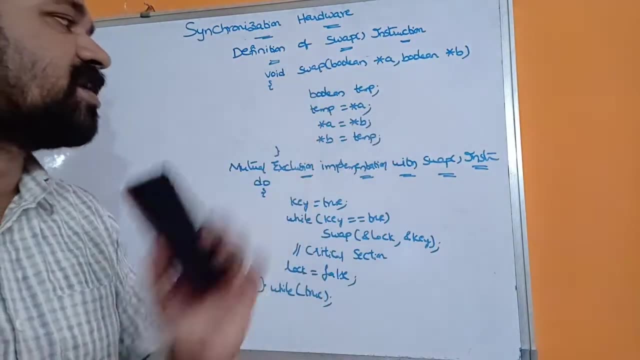 help of a temporary variable. temp is equal to a, a is equal to b, b is equal to temp, but here a and b are pointer variables. so temp is equal to star a. star a is equal to star b, star b is equal to temp. now let us see the code for mutual exclusion. mutual exclusion implementation with: 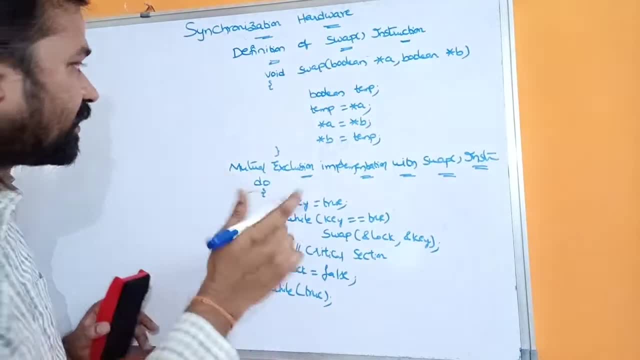 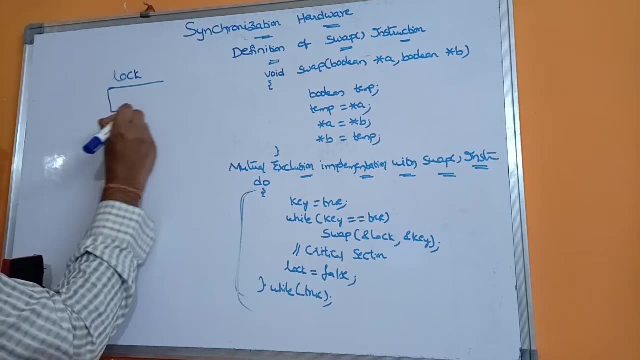 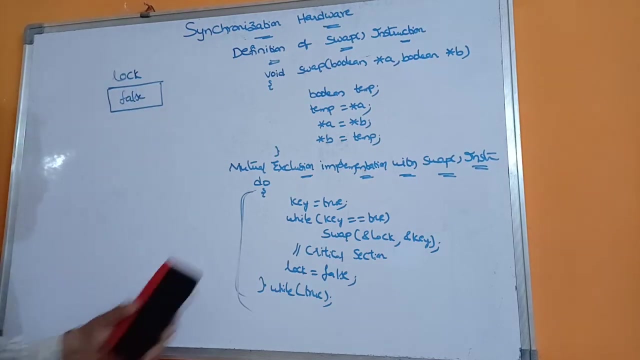 the swap instruction here in each. here. first we use a shared variable, that is lock. lock is a shared variable, so this variable is used by all the processes in the system. the initial value of the lock is false. next to do: key is equal to 2. each process we have. 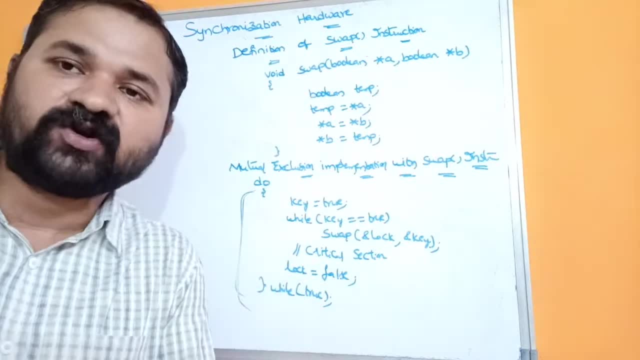 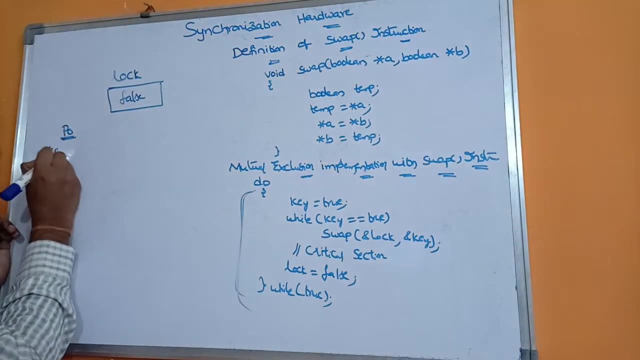 its own key variable. so p naught has its own keyboard variable. p1 has its own key variable. like that, let us assume that p naught wants to enter into the critical section. so first p naught executes the statement key is equal to 2. next y key, double is equal to 2. 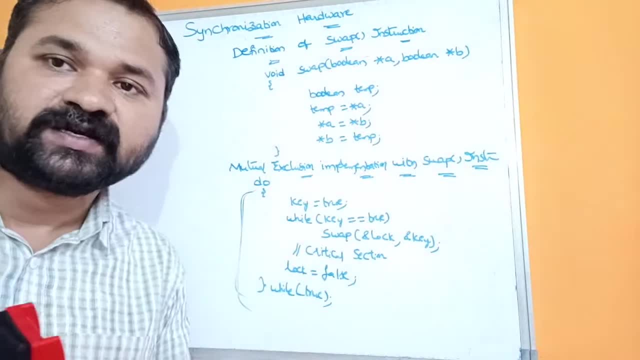 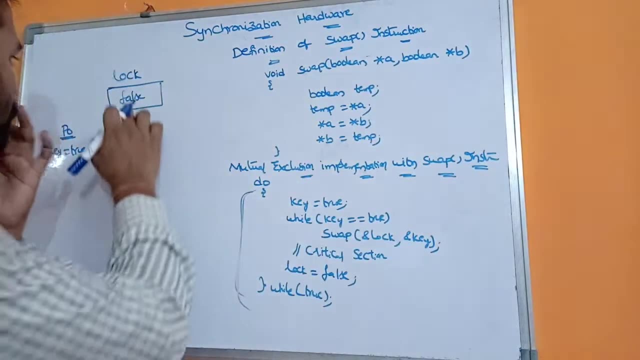 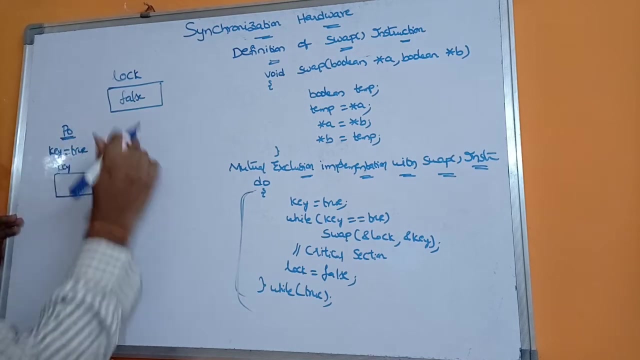 you what is key value? true, true, double is equal to true. condition is true, so this body will get executed. swap of m percent lock comma m percent key here: this is nothing but lock, this is nothing but key and let. so this is key variable. here we are passing addresses: let the address of the lock. 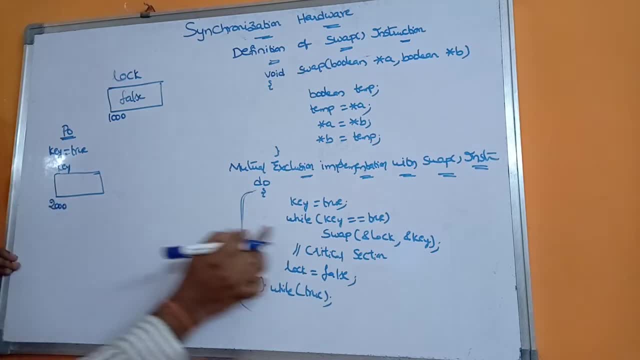 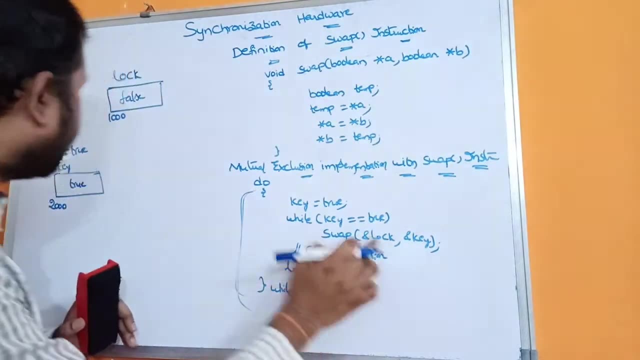 is thousand. various address of the key is two thousand. so what is the value of key? the initial value of the key is true. so swap of m percent lock, comma, m percent key. so m percent lock means thousand, m percent key means two thousand. so this thousand will be. 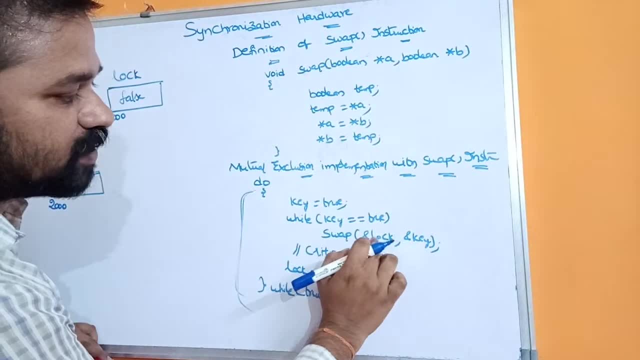 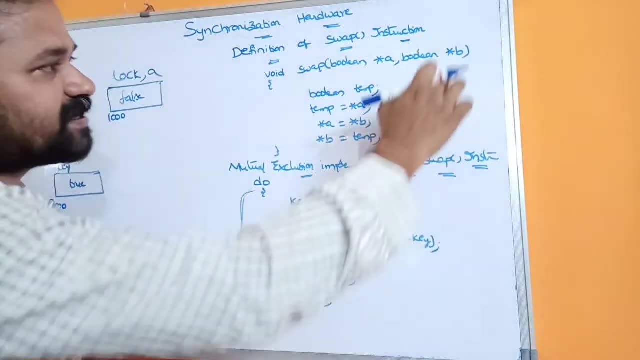 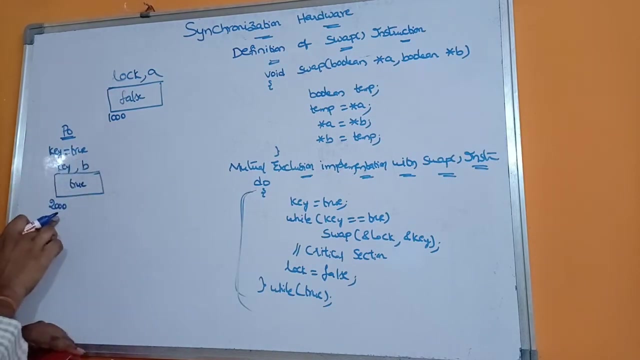 password to a. now, uh, lock and a are at thousand memory location. next, this key address will be password to p. so key address is two thousand, now two thousand, and, i'm sorry. key and b are at two thousand memory location. so if you perform any modification on a then it will be reflected on. 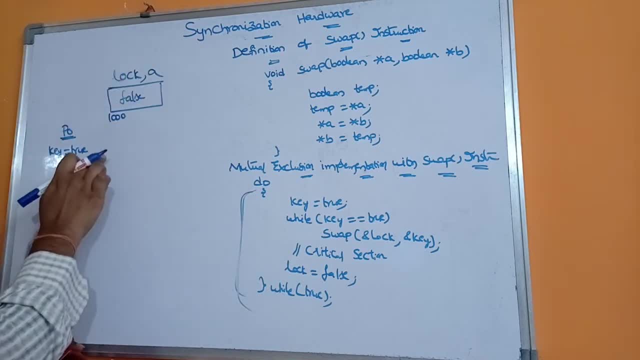 lock. also, if you perform any modification on b, then it will be reflected on key also, because both are sharing the same memory location. so simply, we are performing the swapping. so swap a and b. so what is a value false, what is b value true? so after swapping, what will happen? it will become false. 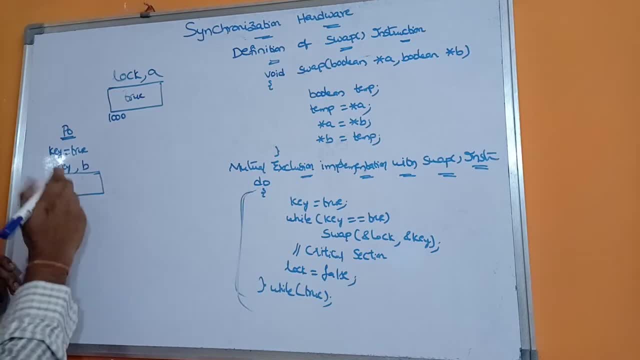 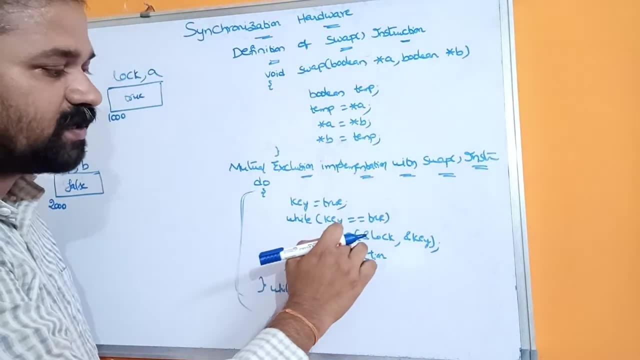 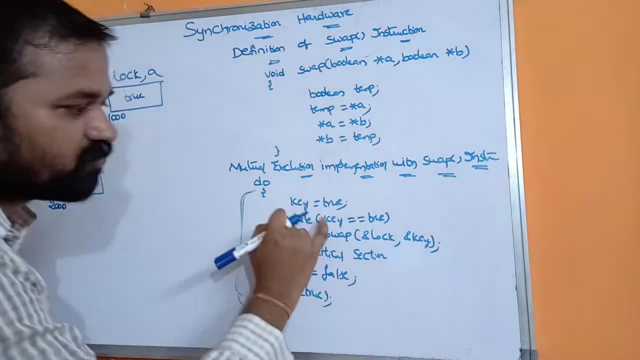 will become true. why? because we are swapping these two. this will become false. so swapping is over. so once swapping is over, control comes to the function. uh, so, once again, control goes to the while loop, while key double is equal to true. but what is key? no, no, key is false, false, double is equal. 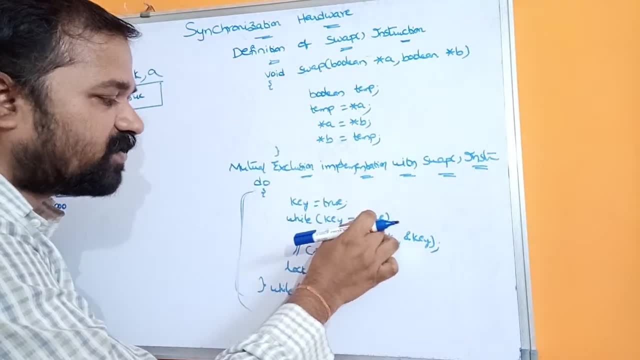 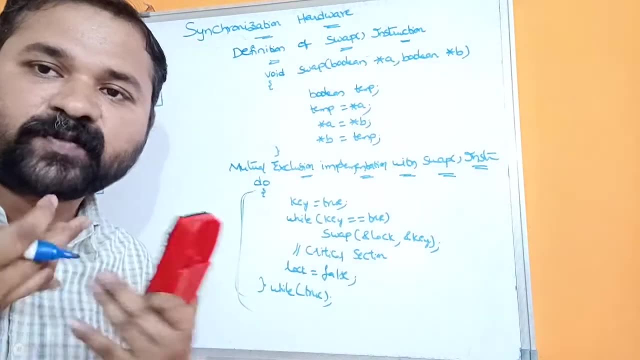 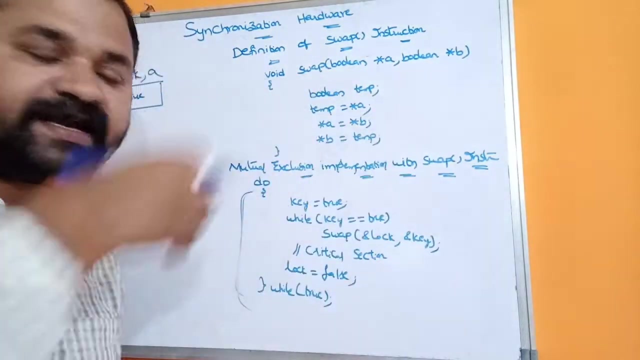 to true. condition is false. so whenever the condition is false, then the control comes out from the while loop. so now peanut process is in the critical section. okay, so now peanut process has- uh, once peanut process completed all its operations, then peanut process comes out from the critical section. after coming from the critical section, it makes the log value as false. so that's. 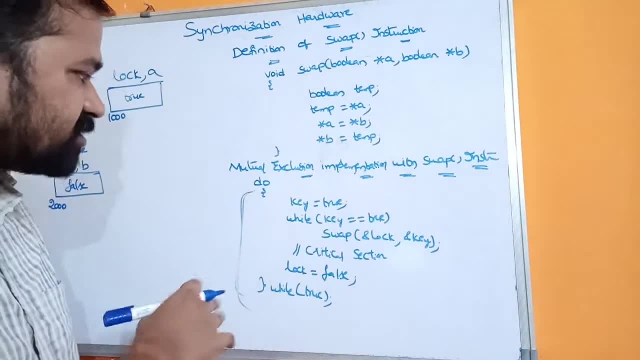 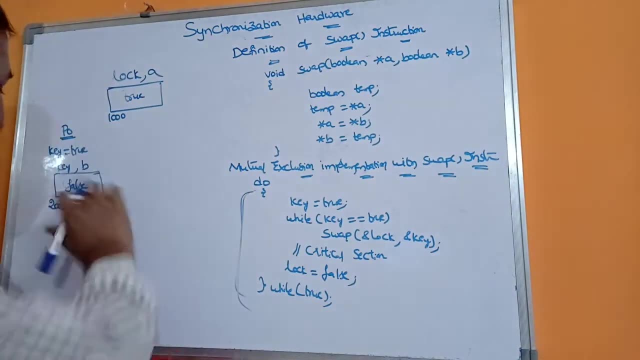 another process will enters into the critical section. so this is the logic here. now let's check whether this code is providing mutual exclusion or not. let us assume that peanut process is in the critical section. while peanut process is in the critical section, let us assume that p1 process. 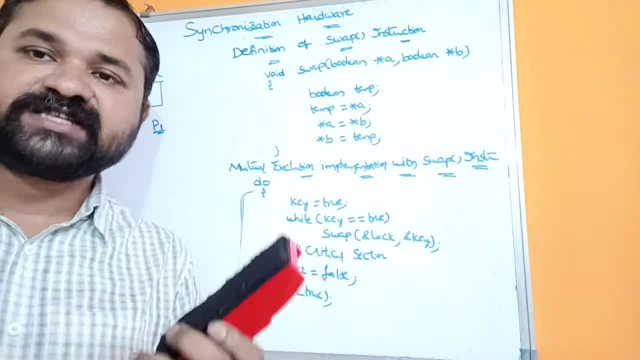 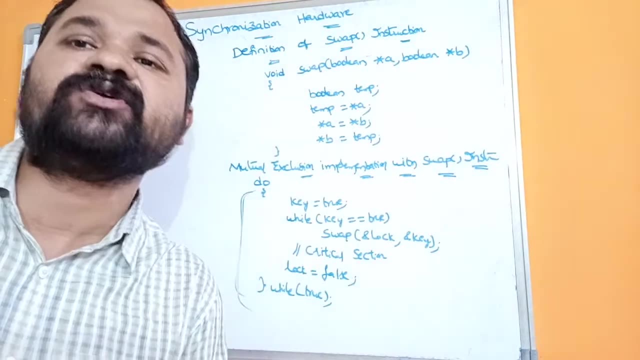 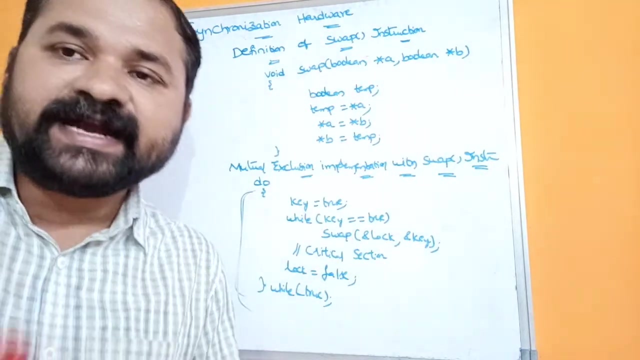 wants to enter into the critical section. uh, we know what is critical section. okay, critical section is the region where one process can execute its execution. let us check whether this i mutual exclusion or not. so we know what is mutual exclusion. at a time, only one process can enters into the critical section. okay, that means one. when one process is in the critical. 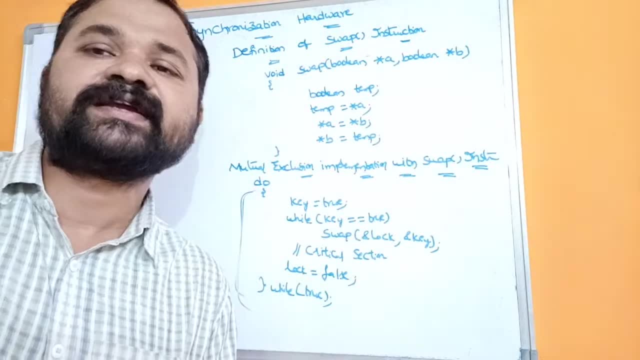 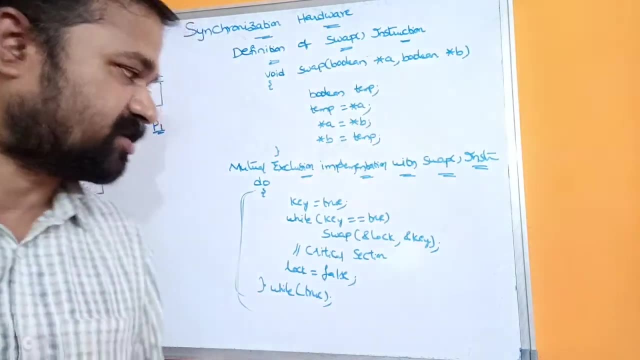 section, then no other process is allowed to enter into the critical section. so when p naught is in the critical section, then we should not allow other processes to enter into the critical section. let's check whether it is correct or not. p1 execute this statement key w. key is equal to 2. here key. 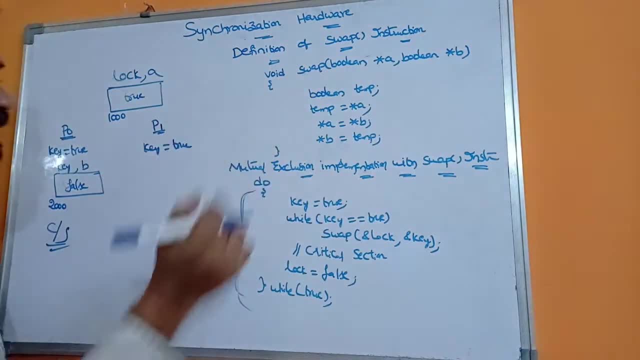 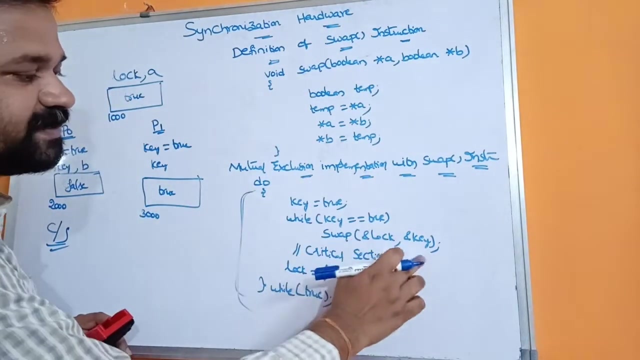 is its own key variable. next, y key double is equal to true. yeah, condition is true, so this function call will gets executed here. key is a local variable, so p1 has its own key variable. let us assume that the address is 3000, the value there is true, so swap of ampersand log comma, ampersand key. 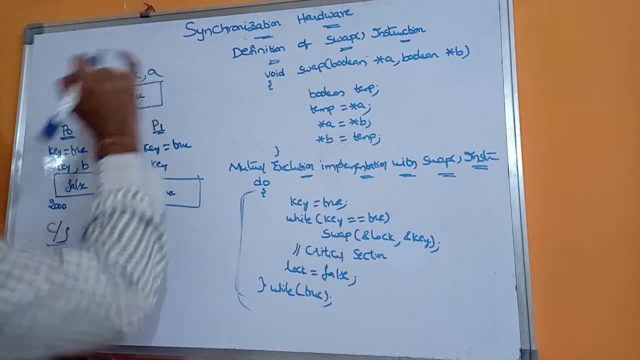 so ampersand lock means what this thousand? so this thousand will be positive to a. so what is log value true? next, the ampersand key will be positive to this b. so now key and b will share memory location. okay, so what the swap function will do. swap function will interchange these two. 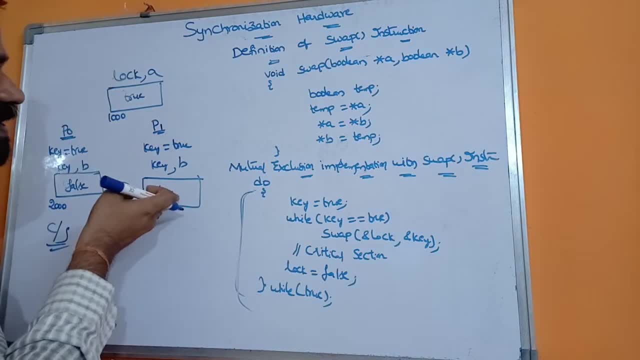 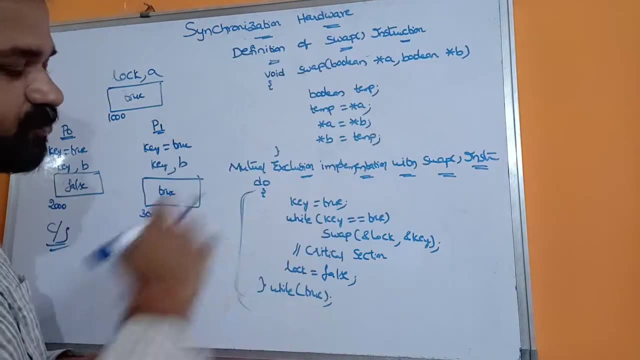 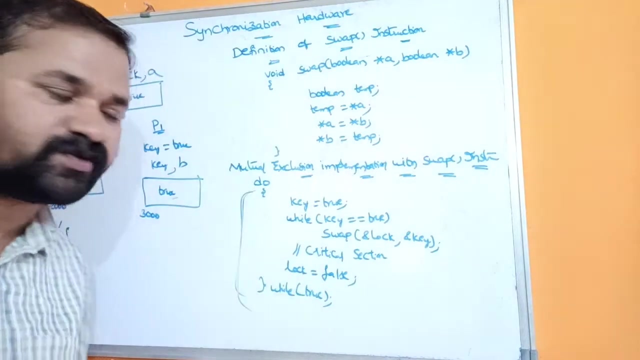 values. here the initial value of a is true as well as b is true. so after swapping also a will becomes true, b will becomes true. so once that definition is over, control comes to the function. while key double is equal to true, what is key true? so true double is equal to true. condition is true. so once 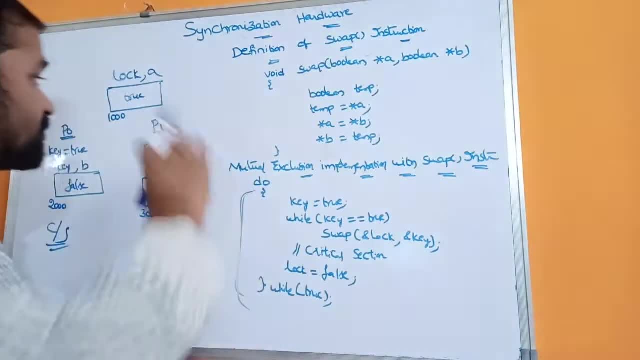 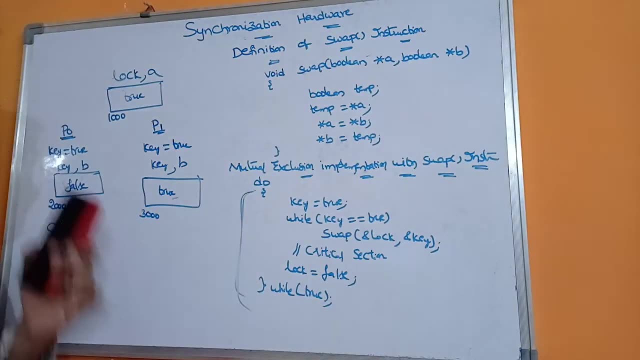 again, control goes to the swap function. so swap function code will execute. so these two will be sample. so true, true will be. so once again, those two values are true, truly. so that means here: p1 process always stays in this while loop as long as peanut process is. is comes out from the critical section. okay, so whenever p0. 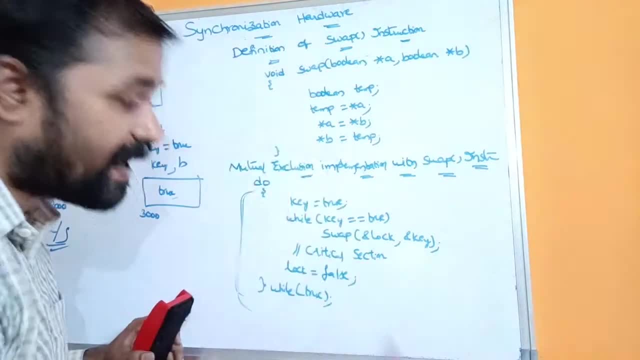 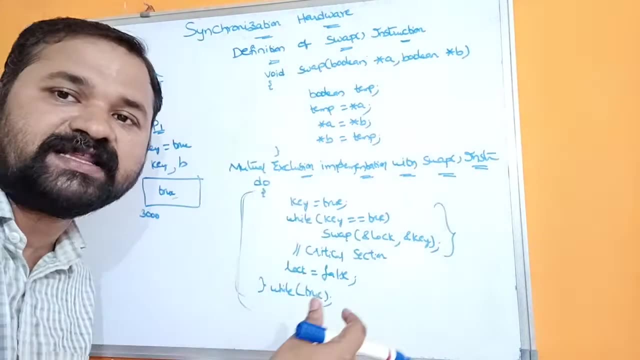 process is in the critical section, then p1 process is not allowed to enter into the critical section. p1 process always stays in this loop only so we can say that this algorithm is satisfying mutual exclusion. and now let's check whether it is satisfying bounded waiting or not. we know that. 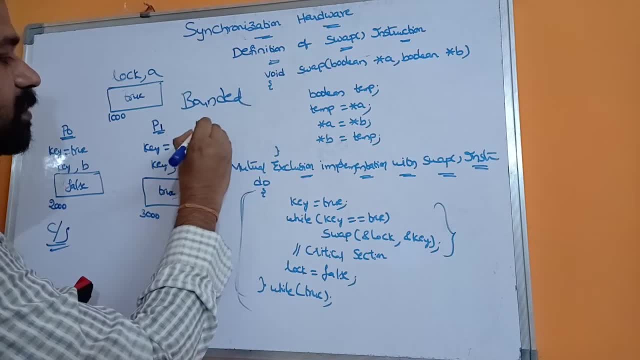 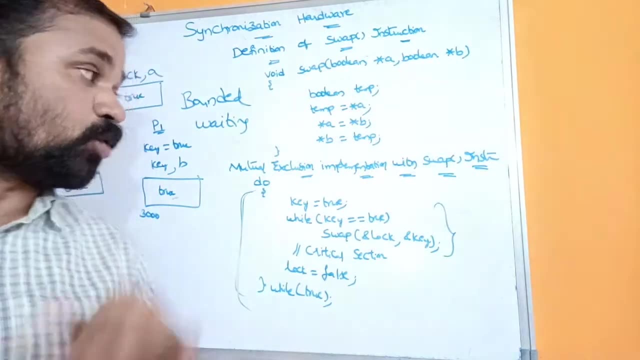 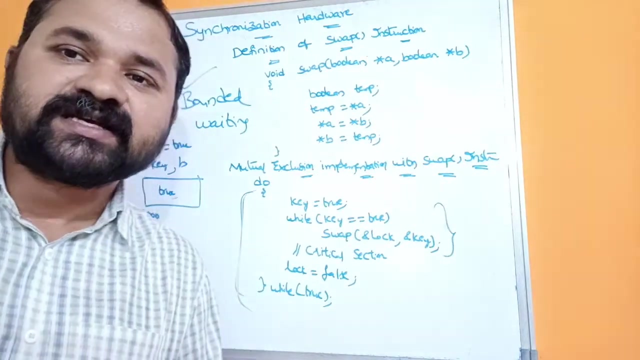 any solution to the critical section problem must satisfy three requirements. first one is mutual exclusion. second one is bounded waiting, whereas the third one is progress. it is satisfying mutual exclusion, let's say whether it is satisfying bounded waiting or not. so bounded waiting means there should be some restriction on a number of times a process can enter into the critical. 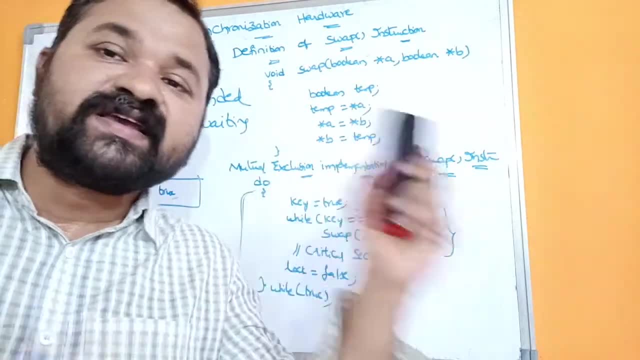 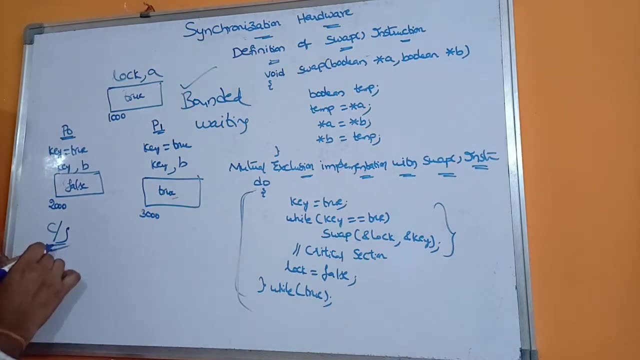 section. so we should not give more chances for a single process. chances will be given equal for all of us. let's check whether it is satisfying or not. let us assume that p naught has completed all its operations in the critical section and p1 is waiting for entering into the critical section.